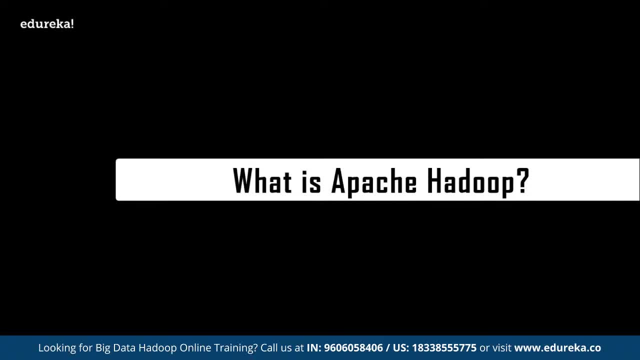 we have added 20% of the data in last two decades. So you can now imagine how much of data is getting added year on year, And especially last five to eight years have been significantly enormous amount of data getting generated. It can be in multiples. So the data growth rate. 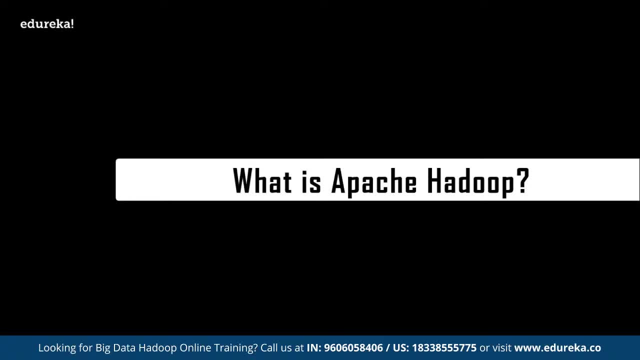 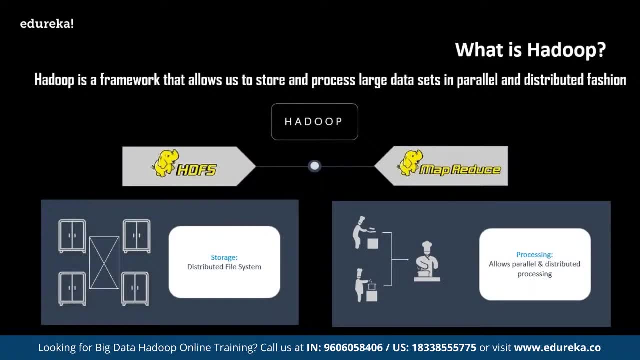 is roughly around 600 to 800% year on year. So, with this much of data coming in, we need a framework which can help us to collect and store. So Hadoop, in nutshell, is a framework that allows us to store and process the large data sets in parallel and distribution fashion, which means 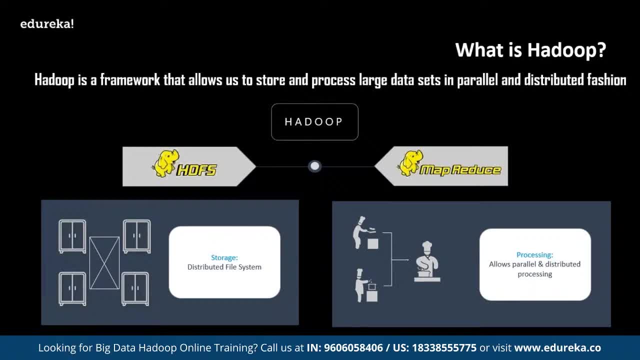 you might be seeing what is happening On your social media sites at any given point of time. the Facebook or WhatsApp have more than billion parallel users who are doing a read, write or post activities, which means they will have to enable all the three things in parallel, which means the data collection, data storage data. 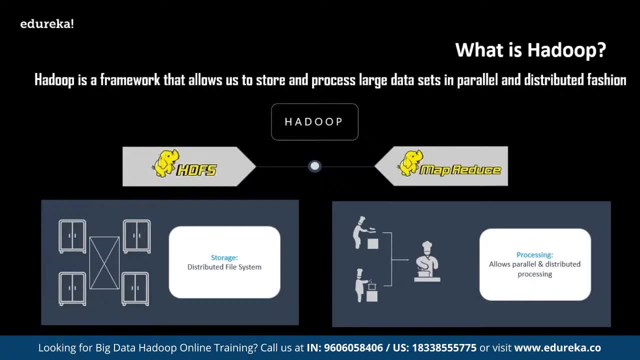 processing, which needs to happen To do that particular things. in parallel, you need to have a data collection, data storage, data processing, which needs to happen. Hadoop comes very, very handy, So this helps you to do the storage in a distributed file. 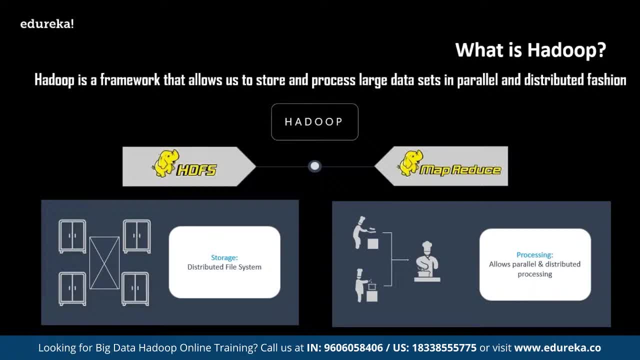 environment, and MapReduce helps you to parallel the process, the data parallelly, and distribute the processing, which means you don't make load centric but you distribute the load so that at any given point of time you are not really having any challenge that way, 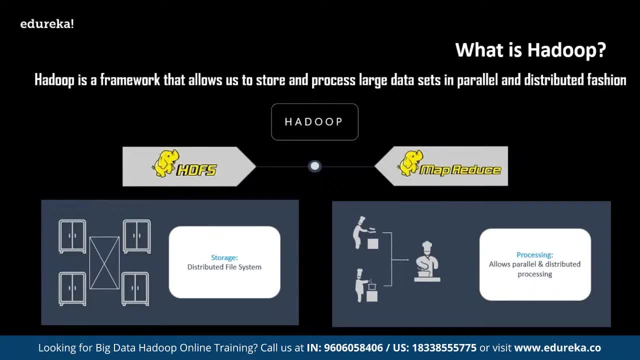 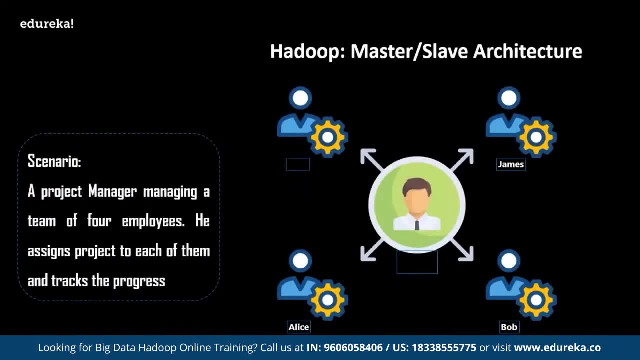 Hadoop framework allows you to store and process large data sets in parallel. And if we have to see a scenario, what happens? basically, if you see this: a manager managing number of four people. he assigns the product to each one of them, which means that's what happens. 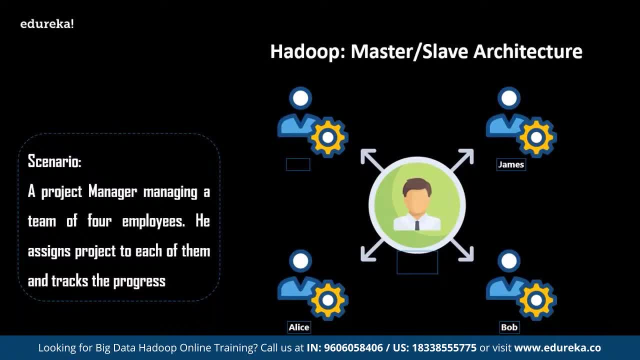 in a typical project management, which means somebody are working in a front-end application, Somebody are working in the middleware application, Somebody are working in a back-end application, Somebody is working with Integrating all of this particular things. This is basically what we get to see in a MapReduce application, which means you are getting your inputs. 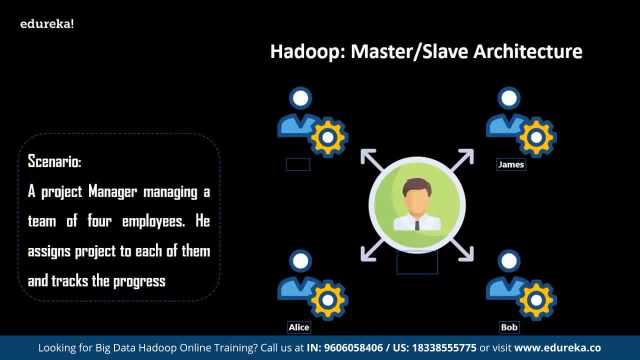 from multiple sources and parallel processing is happening. and then the manager, whoever is responsible for the project, who is your, you can correlate it to your Hadoop framework. He is the one who balances the work schedule, manages to see How exactly the work can be distributed. 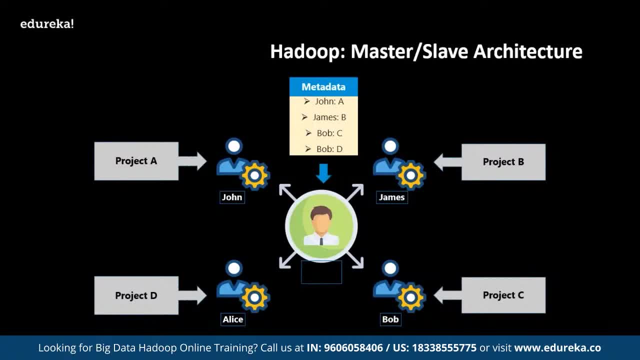 and then he makes what? all the individual or small activities which each one of the resources perform. he tags them. So, for example, John from project a, James from project B, Bob from project C and Bob from project D are doing in silos their activity, while 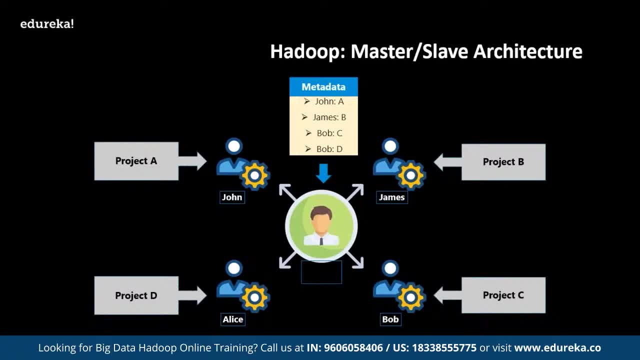 the manager is working in parallel to make the things happen that way: Large activity at a given time in chance. You can also for a minute We can say it is basically working against the time. The reason why I say this is basically: at the same time multiple heads are working, multiple resources. 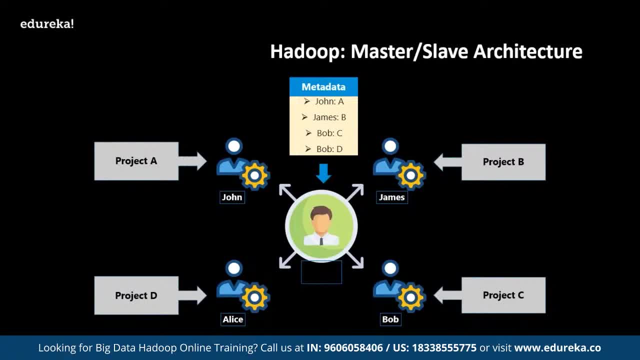 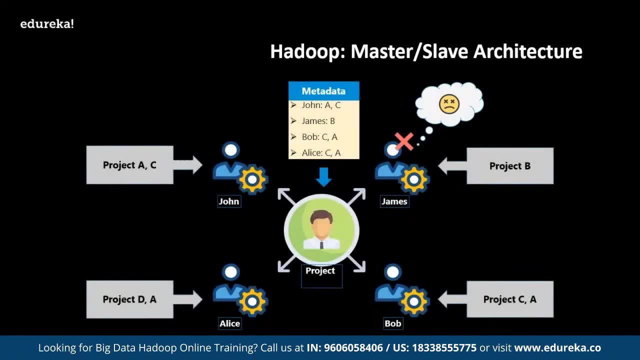 are contributing to their particular task. that way you can make the things happen. So once this framework is happening, imagine if there is any downtime or somebody falls sick, then that particular reassignment or reorg is done by the project manager. So basically there comes your coupling, basically. 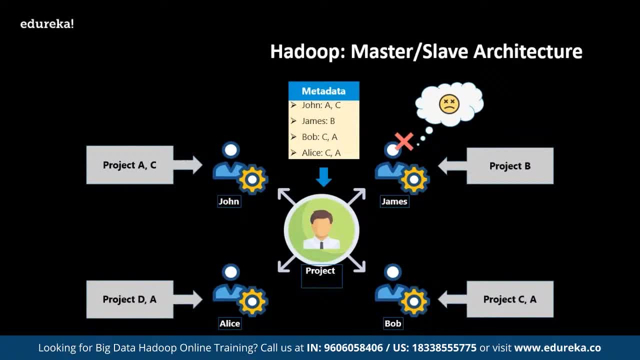 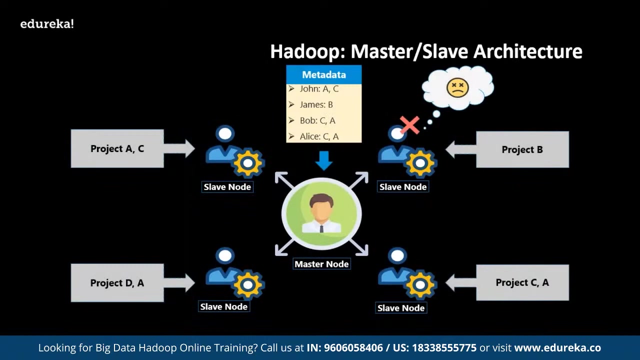 you then re or your thing. So if you see project TNC, John gets to do, project D and A at least gets to do and James was replaced with somebody, person. So that management of activity is what happens seamlessly with your framework, This big data framework, saying that that particular thing. now 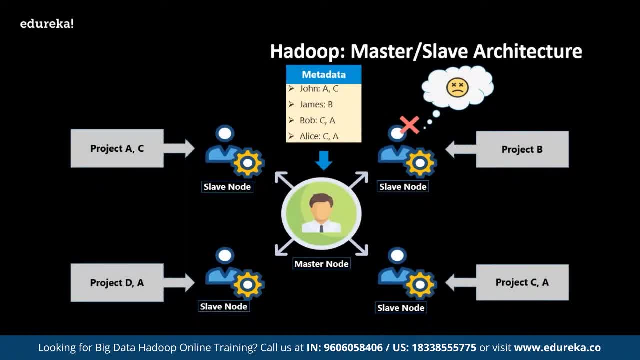 if you have to see technically, this is the master node. who is the project manager becomes the pastor node. all other resources who are enabling the final dedicated activity becomes the slave node. So you have the slave nodes, You have the master node, and master node usually tries to mimic between what is happening versus. 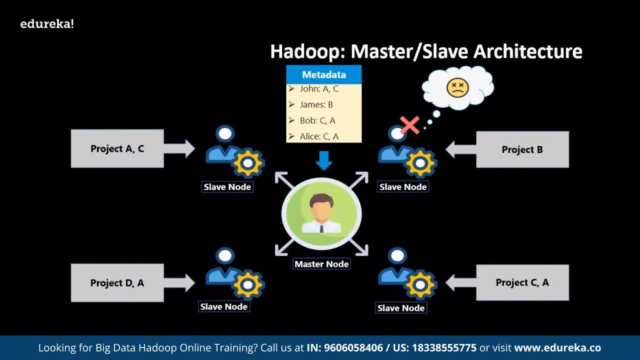 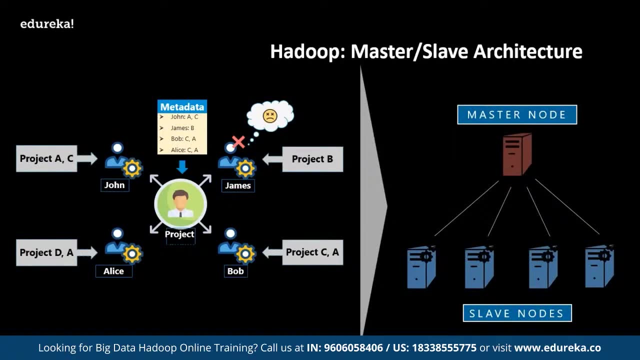 what is not, And then gets going this way: You are master, slave, architecture gets addresses. Then if you have to see the next thing, basically what, what happens here? we are trying to show that pictorially. So this was with regard to the project manager, with regard to the resources. 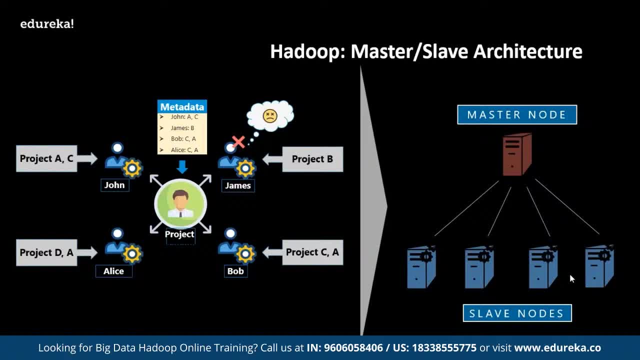 and the same thing. it becomes a master node with associated slave nodes and it's a bi-directional information transfer between the master node and the slave nodes. that way whatever is happening at the slave nodes intern gets reported through a master node and master node keeps the track of all the parallel processing this particular activity. 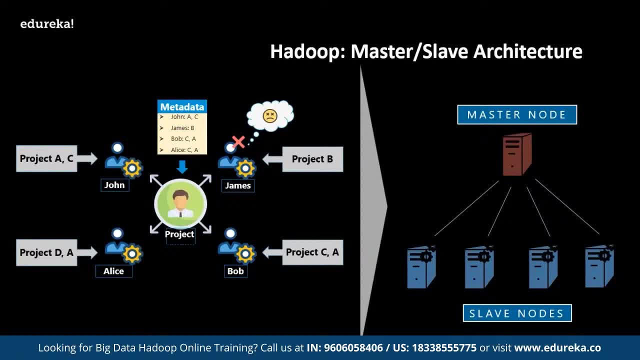 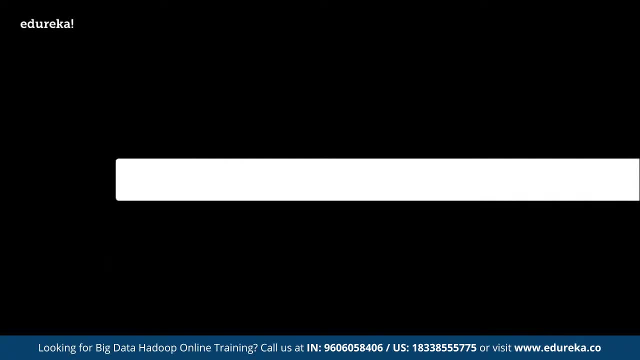 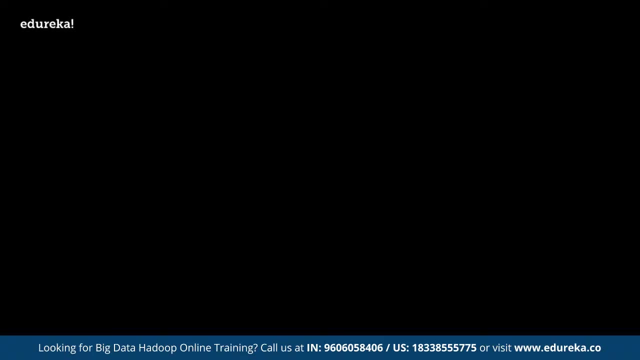 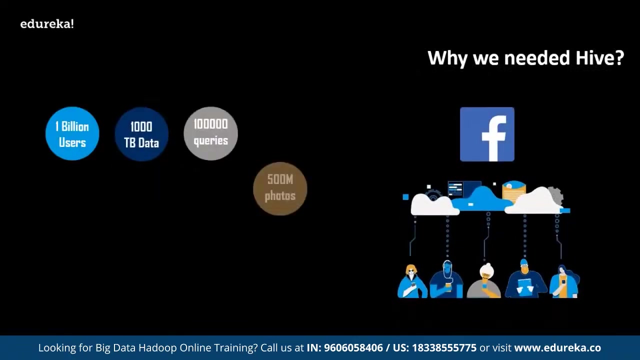 of managing large data sets with parallel processing becomes your framework of Hadoop or big data. So with this we will have to see what is the need for Hype, for which we will have to see what exactly is the whole benefit of using hiding. So here, if you happen to see some numbers in terms 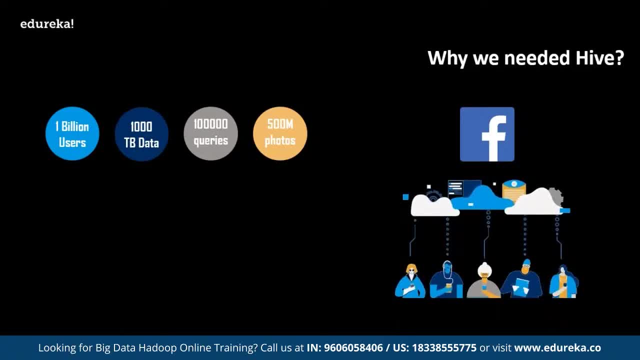 of how much of data is getting generated. So, for example, on a Facebook, the number of users, a billion users, 1000 terabyte of data, 1 lakh queries, 500 million photos. So we all know, with every increase, or rather with very latest models, 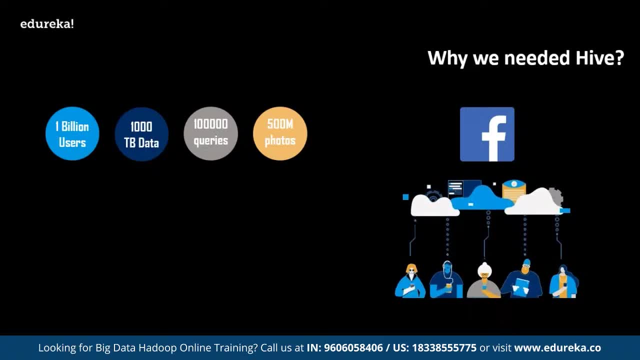 the megapixel of the cameras are very high, and high megapixel cameras are usually of large space, which means their Excel is very fire. So with this much of data getting loaded and you would have all seen, Facebook is a bottomless page. you keep going. 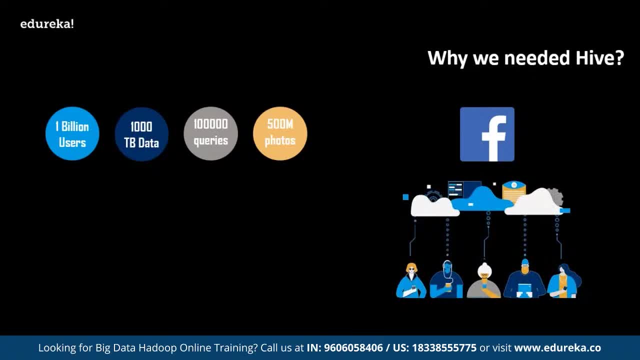 It doesn't end, which means it's continuously Generating data. this generated data has to be stored and parallel processing has to be done. for this particular thing, You will have to have a framework which is continuous in nature, at the same time, which is not redundant and which does not break. 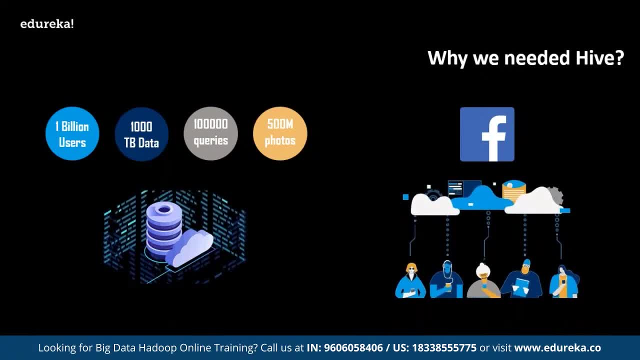 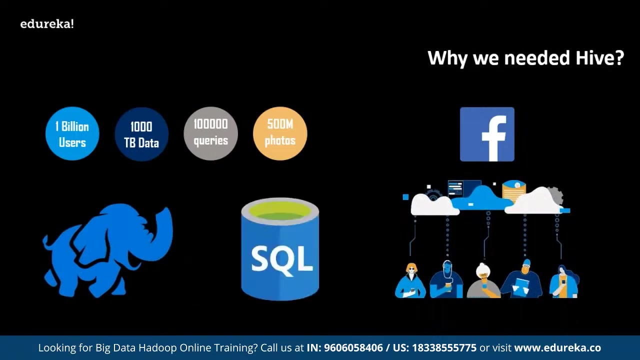 and if it breaks, the reassignment from the master to slave has to happen seamlessly without in during the user experience. So to do all this particular things, we need a placeholder which can help us to see how we can do this. So that's where Hadoop with hive comes handy. 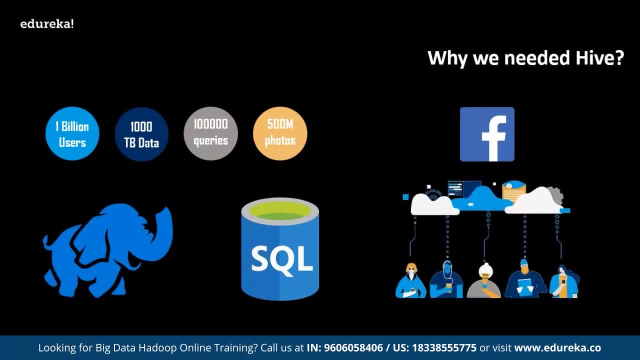 So, basically, the databases can be anything. It can be an SQL database, It can be an Oracle database, but the data quotient which is getting generated is very, very large. when that large data, questions have to be admired and admitted, you need to do the things. 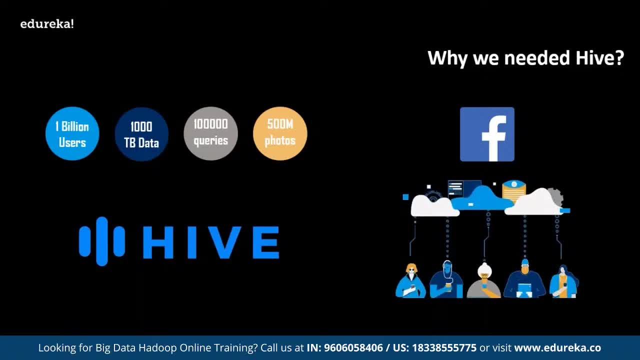 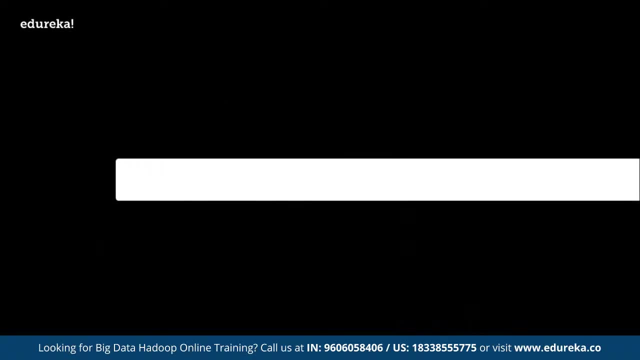 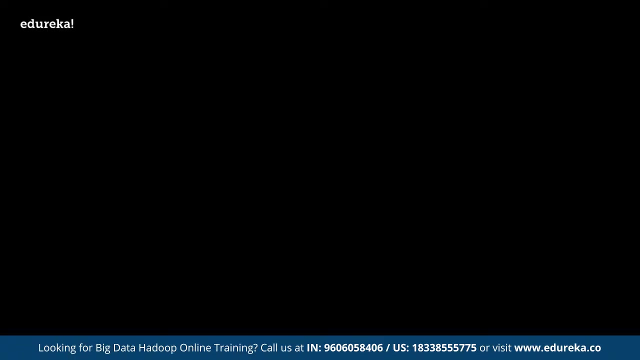 with an additional enabler, which is hive, so that way you are using your Hadoop with your hive to make the things as seamless as possible. So if that is hive, then what is Apache hive? All right, So let's try to see what is Apache hive. 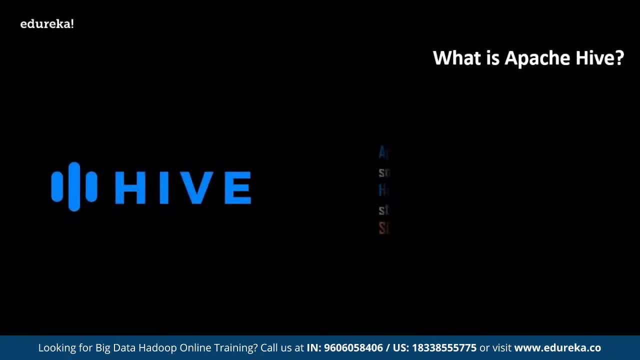 So if you have to see what is Apache hive, basically Apache hive is an open-source software built on top of Hadoop to provide easy data storage and analysis in style of a scale, So most of us would know the database. So it is a simple RDBMS relational database management system. 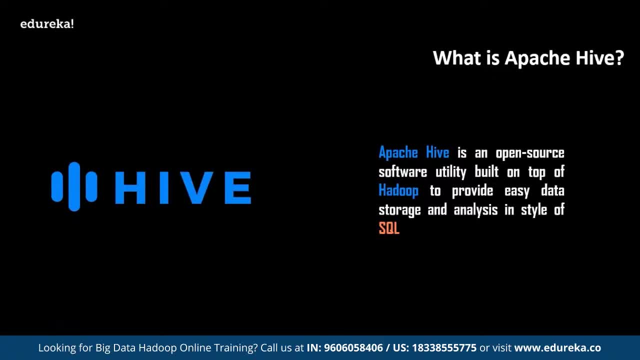 So what? what is the good part of a relationship data? Relational data storage mechanism, RDBMS. The way we can write the data, change the data, retrieve The data is through simple queries, which means we have been we have got used to the SQL approach. 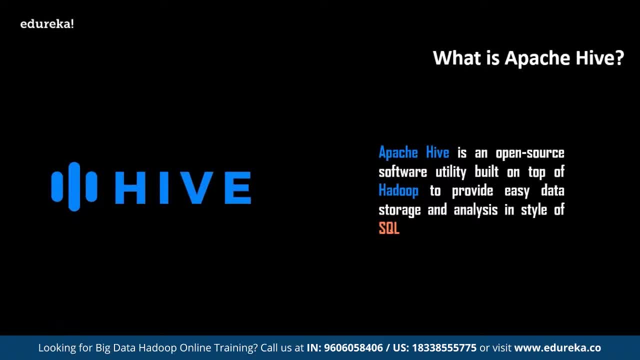 so heavily that this can be done in a same fashion. So that way, Apache hive is also an utility which sits over and above Hadoop, Which can provide easy data storage and analysis. So storage is the right function. analysis is the read function, basically, which we can retrieve from the data. 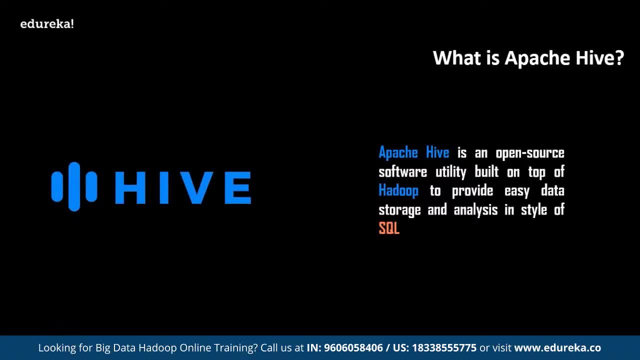 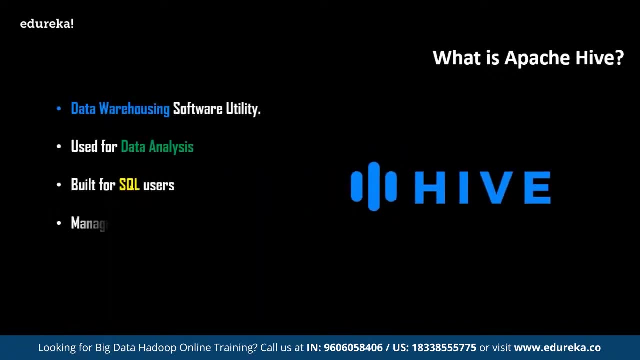 which is stored in the final database. that way, hype is very, very heavy activated in terms of how you can really write and read the data using the Hadoop framework. So that way, hive has become significant in terms of data warehousing, used for data analysis, built for SQL users, managers querying 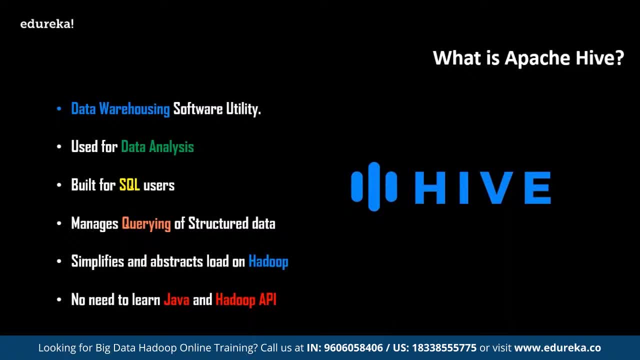 structural data simplifies the abstract load and no need to learn Java or Hadoop ABA, which means basically your request for the details becomes from a user friendly perspective. You don't have to really do what exactly, or rather how, a technical person can do. a relatively non-technical person can easily handle. 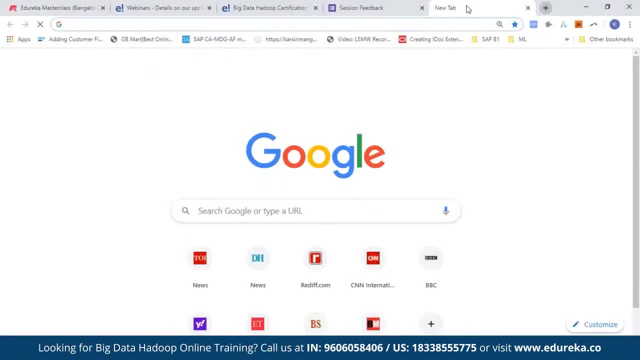 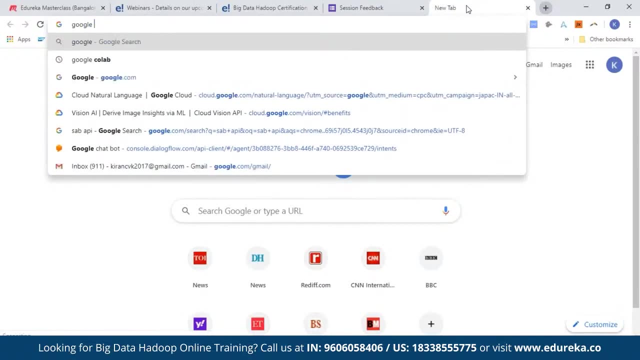 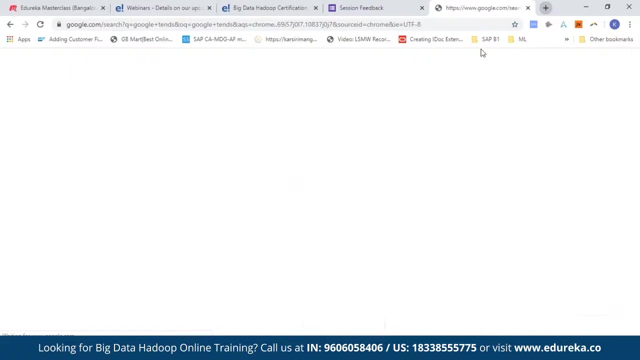 So if you have to go ahead and see the usage, So one thing is basically, you can always go and see how the world is adapting for this new technologies. You can go to Google Trends, So this is the website which gives you how much of searches are happening in what geography. 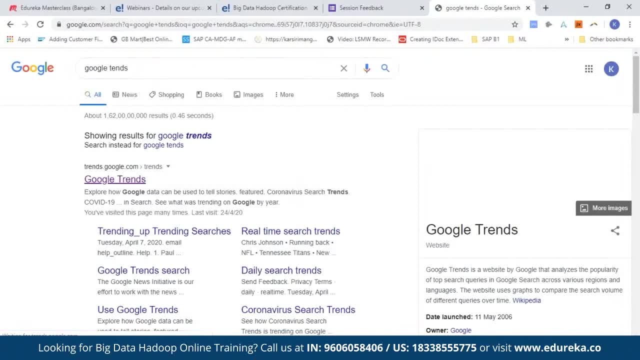 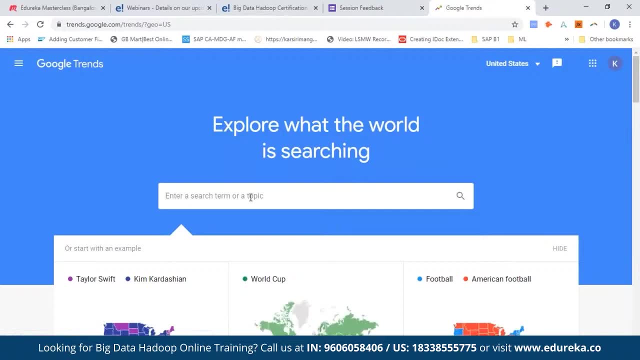 for what kind of a keyword? So if you, if I, go to Google Trends and type the hive or Apache hive, let's get to see the real Time. what exactly is the trend for last five years? So if I say Apache hive, 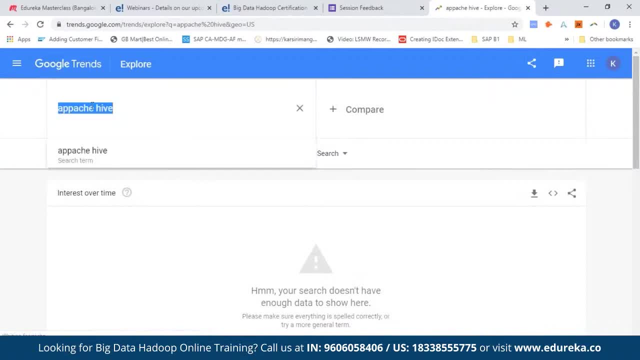 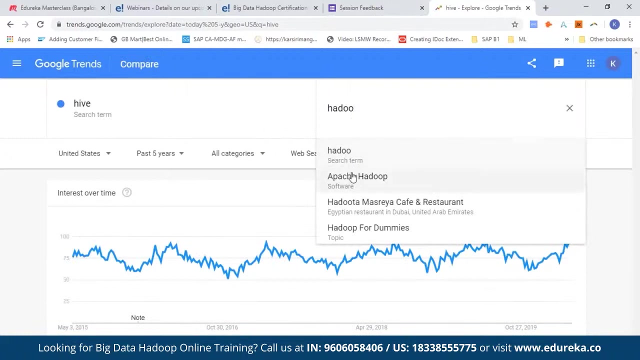 so if I select or leather, let me make it hard- or, And if I select for last five years, and if I also compare it with a like-minded thing like Hadoop Okay, Apache, Hadoop, Okay, so you get okay. This is basically. 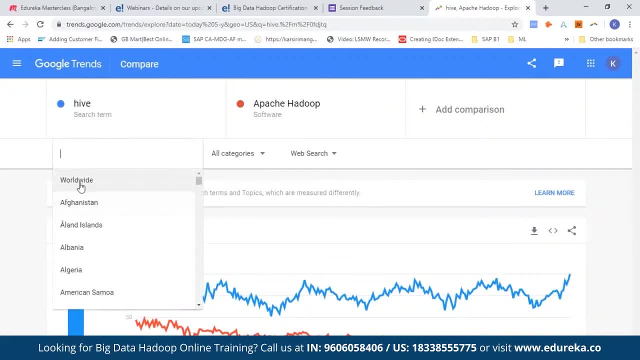 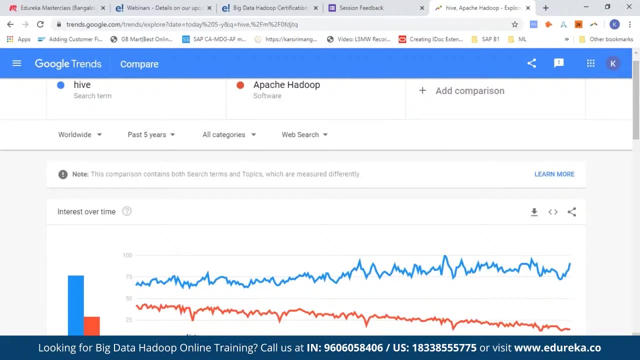 I have selected only for United States. if I go here and select for worldwide, you get to see in related to a Hadoop, The hive has relatively higher searches in last five years And if I have to come down here and see the timelines. basically, this is how it works. 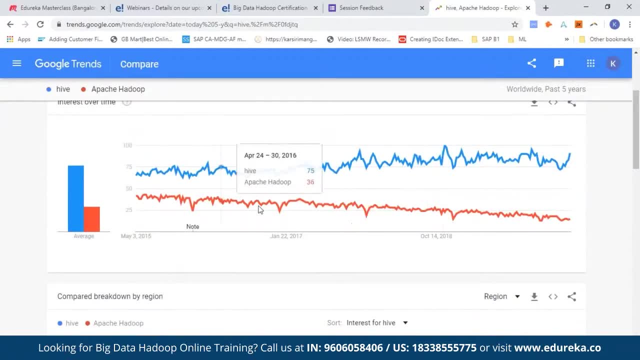 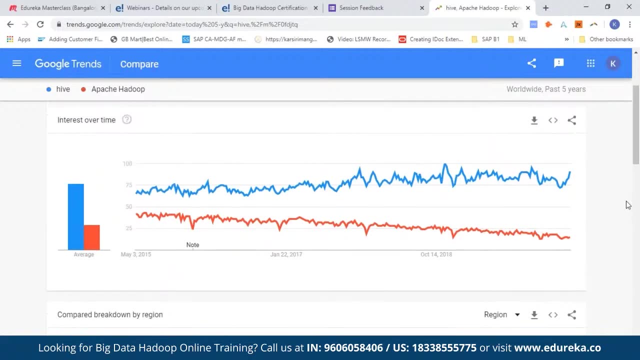 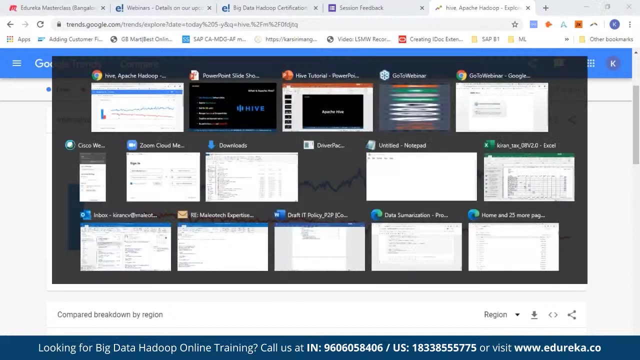 Okay, let me go little. Okay, if you see here, from 2015, the hive basically has much More significant searches. So when do people search? when they are using or when they are technically trying to understand this set? So Google Trends clearly indicate the higher adoption rate. 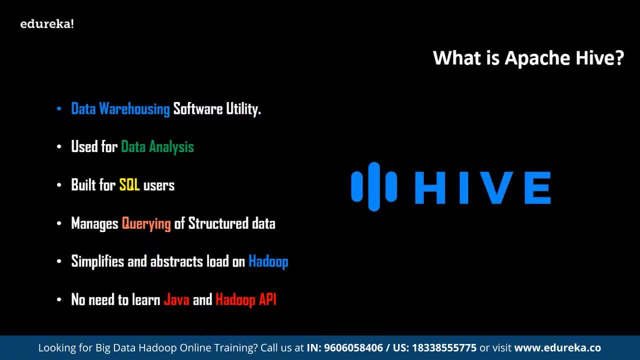 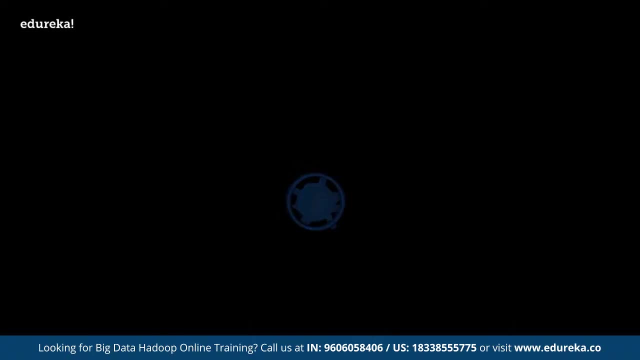 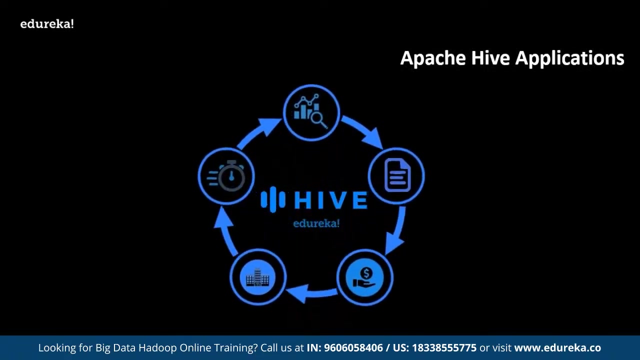 because of that user flexibility. So, like we see, these are all the placeholders What are where Apache hive is used. So, saying this, let's see what exactly is our applications of hive, So where exactly We use Apache hive. So there are endless, or rather so many high applications. 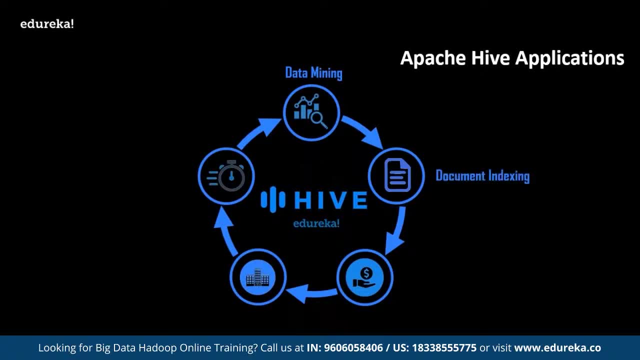 which you can think of, which is in data mining, document indexing. So predominantly, imagine about a cloud server which is of a large storage and their victory will become such a challenge. So until and unless you don't do your document indexing, you will not be able to address this and predictive modeling. 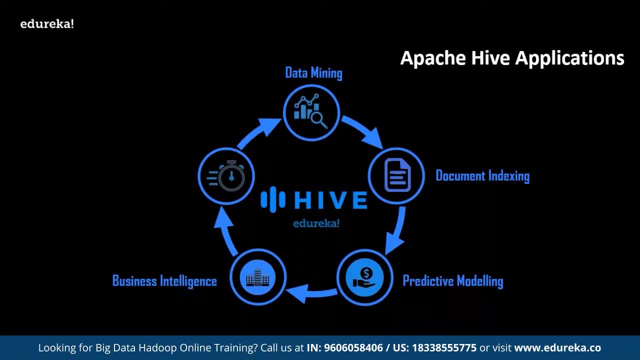 which is used in your data science and machine learning concepts, Where you will have to feed in the data which can be consumed for your downstream applications. there you use your hive and then you get to your business intelligence. So what is business intelligence predominantly trying? 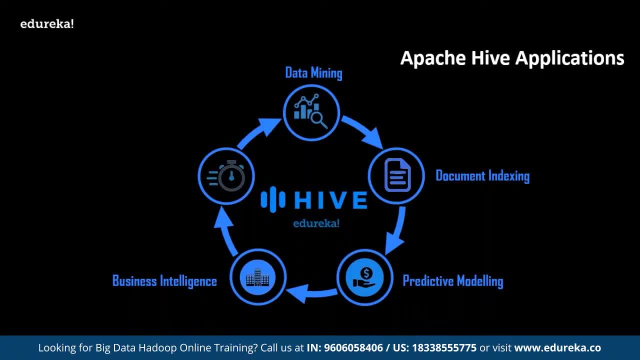 to enable business to take appropriate or amicable decisions for the given options becomes your business intelligence, which means the options are ample. today's business decisions are very complex, So until and unless you enable a tool which could consume All your data and influence, you will not be able to do this thing. 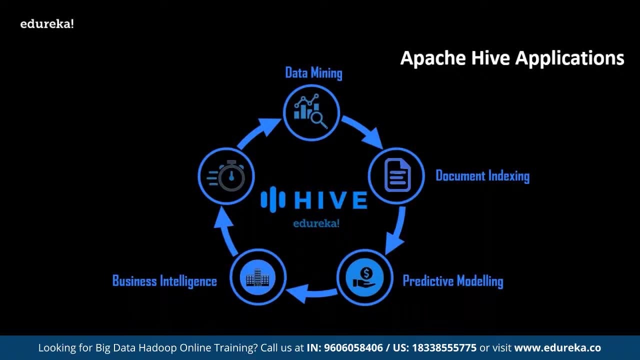 So that's why, even for business intelligence, you happen to use your hive applications, then coming into log processing, So we all know there is a monitoring for all the activities, which are 24 by 7. probably it can be a simple banking project, or it can be your social media. 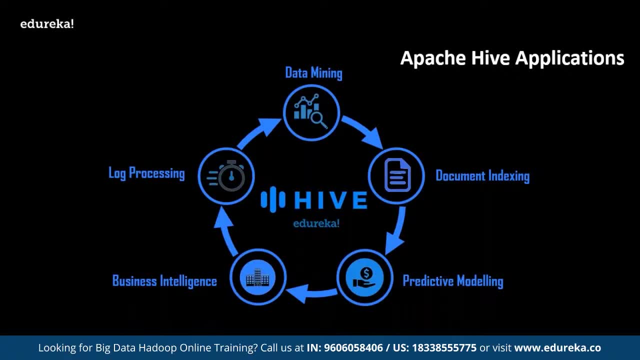 It can be very ATM services. It can be your mobile phone services, where the world is becoming into digital Transformation. your log process, log collection, is one of the biggest task and whenever there is a log collection, the log processing has to happen. So for log processing with such a large amount, 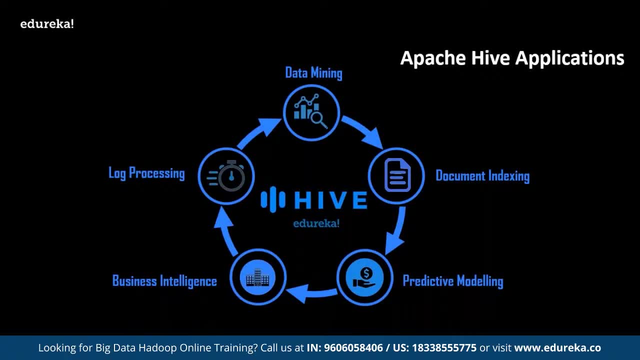 of semi-structured data. you require an application which can do all these things, very, very helpful. So you get to do and see all this particular things for your log processing. So some of this are at a very high level. data mining, We all know, right dominantly. 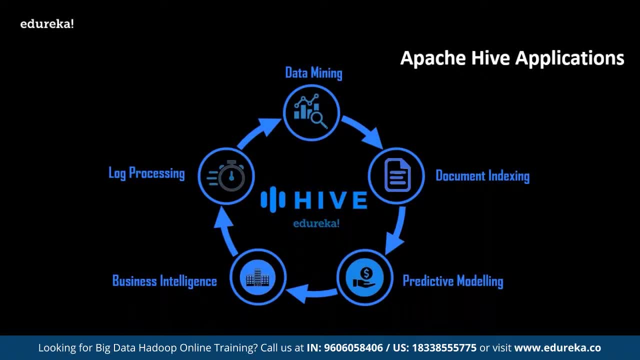 It is about. there is a humongous amount of data, but you just cannot consume all the data. You will have to mine what is needed. So you have to do your data mining. for that, You use your hive applications and get going. 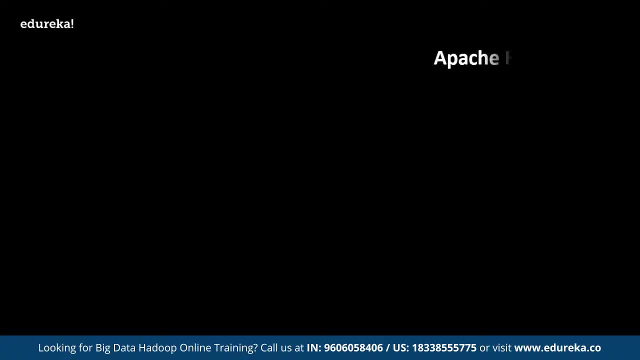 So then, coming to some of the features, So what exactly five with such a high relevance? So if you happen to go and see the SQL type queries, because we already discussed it- has a very close association with the database concepts. So SQL type queries helps you. 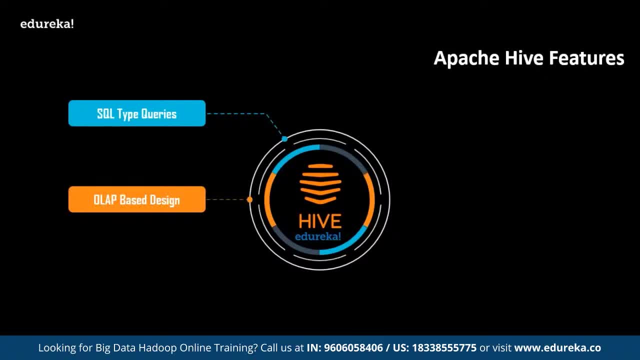 and then your overlap based designing instance. The way the structure is designed makes very well, or rather self-contained, self-sustained- query builders, So that's why it is much appreciated and much used. and with regard to the latency, in terms of very, Very to result, you have a significantly lower latency rates. 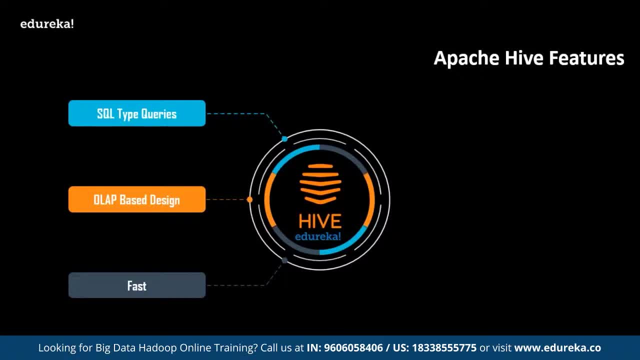 So making the whole application very, very fast. then scale up. even Facebook was created, probably they would have never thought that they might have to process 1 billion users data at any given point of time. forget processing 1 billion data at any given point time. They may not even have thought. 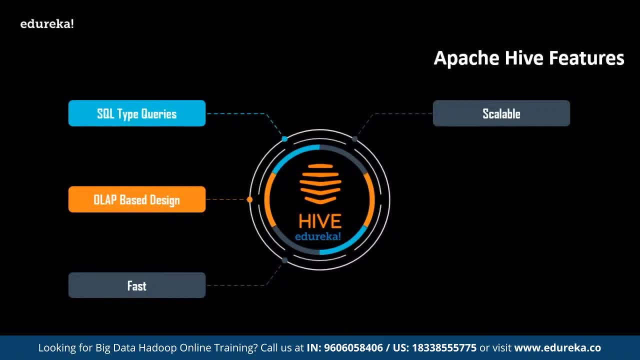 that there might be 1 billion people on their right. but for that kind of things you will have to plan a system which can be easily scaled next extensible right. So basically this goes very well tagged with your scalable So whenever you have to extend it and connect. 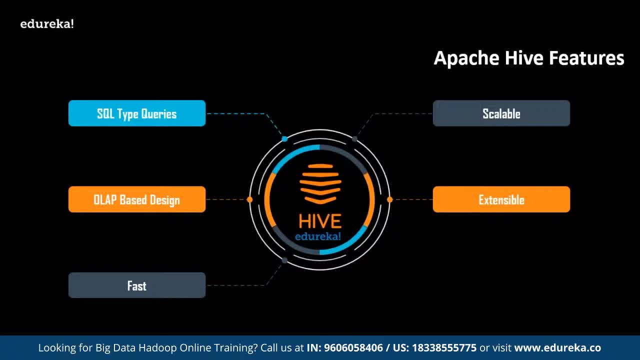 with other associated things. So probably, if you have to see the series with five years or eight years back, Facebook was only an application which was available, a browser based. but today the app traffic has overtaken Then the browser traffic by three to four times, not even percentages- 300. 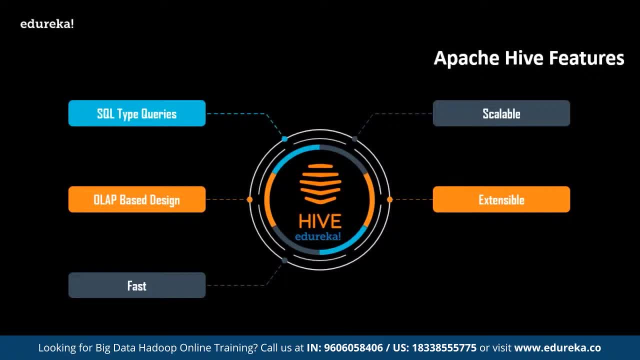 400 percent, which means if you are build an application which is only browser based and not compatible with your app based, probably it would have been a big issue stopper. So that way you will have to make things which is extensible and high supports it very well. 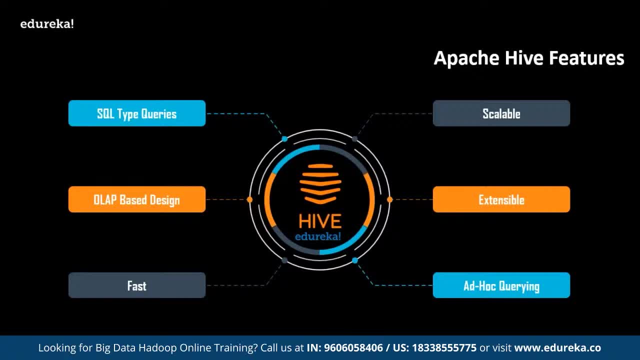 and ad hoc wearing, because there are two types where you can build for regular queries, for your repeated Reporting, but you will need an tool which can help you to mitigate the ad hoc query So that is well structured and well supported using your Apache hive. that way you get. 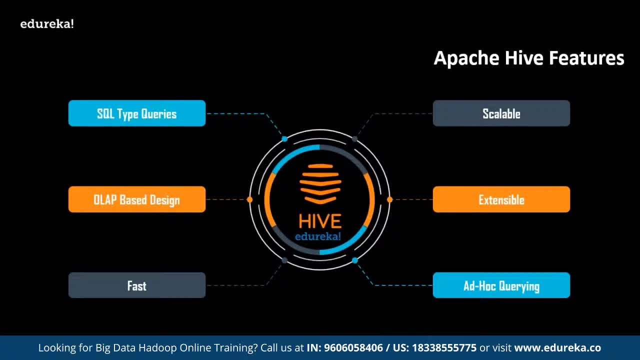 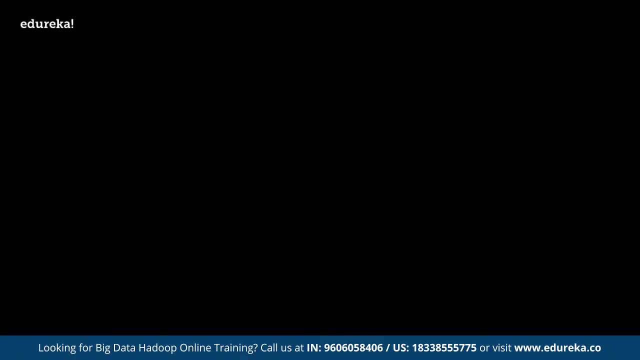 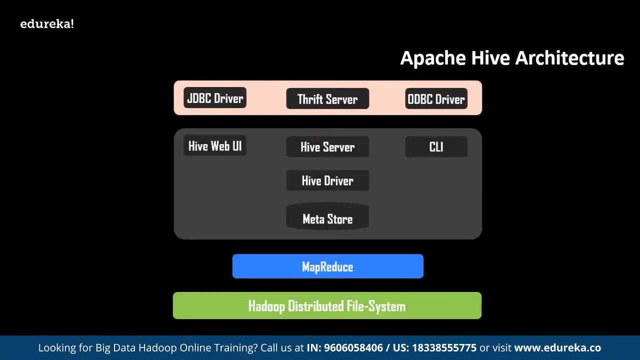 to see and do the things. So basically, this six factors make high very, very advantages in terms of why, what, how, questionnaire. then let's get and see the Hive architecture at a very high level. So basically an architecture looks at this three stages. So you have the lowest level, Hadoop distributed file system. 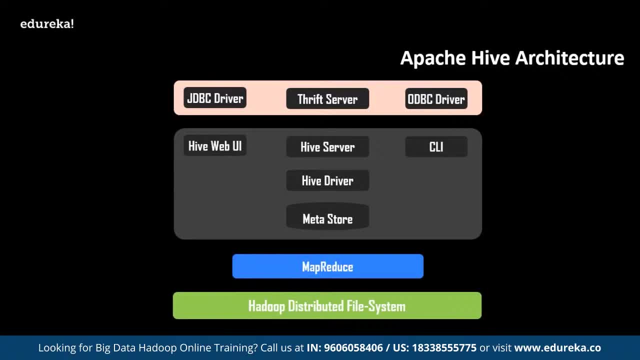 over which we use the MapReduce, using the MapReduce techniques. Then you have all your external sources, like your web UI, the hive server, hive driver, Metastore, CLI, all these things which your JDBC driver or the trip server or the ODBC drivers sits on this. 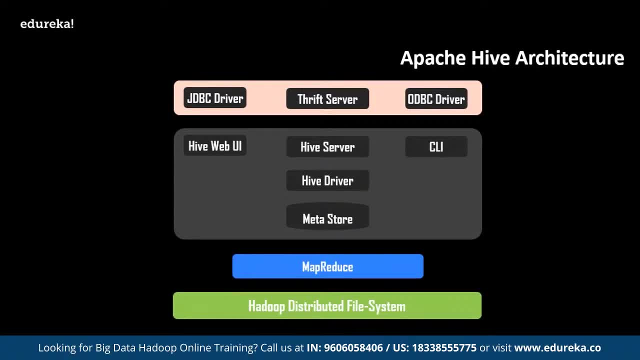 So basically they are interlinked in a fashion which can make things much easier. So it is a straightforward approach. many times You can also call it as a four-level architecture. So the Hadoop file system is your underlying things, on which you re-orchestrate the whole high framework to make things. 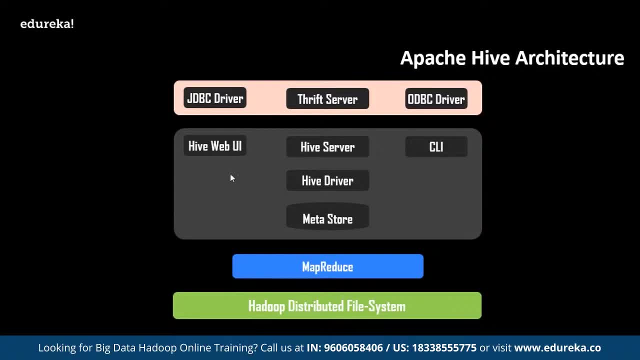 as seamless as possible. So trip server is a server which can integrate with your downstream applications of your web UI or server and, if at all, it has any upstream applications like external things. it can be as simple as an Android app and our mobile iOS app. 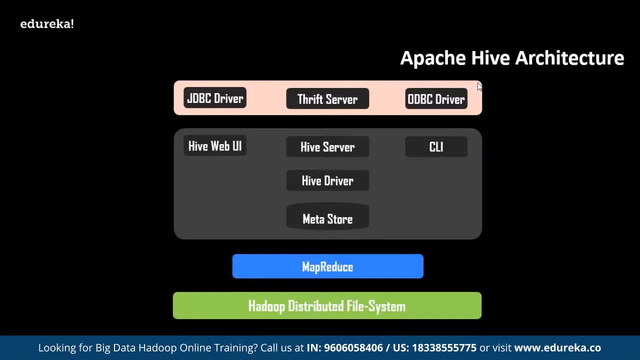 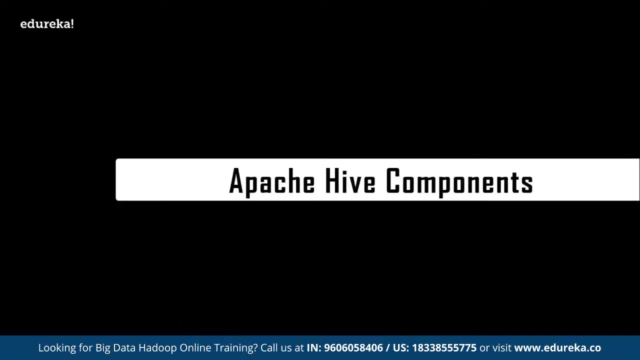 So this balancing the trip server usually accommodates, so that way you are covering the whole framework. Okay, So, saying this at a very high level, is the architecture of Apache hive. So with this, if you have to go and see what is, the components which are associated. 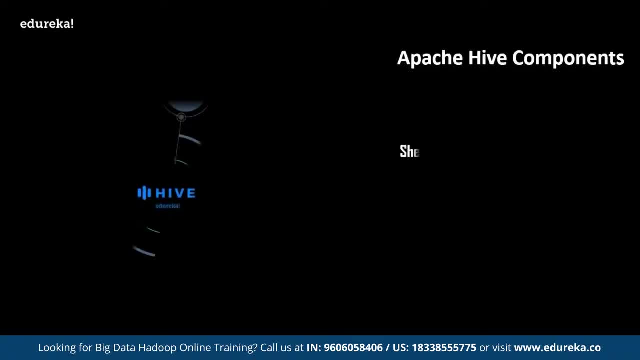 So if you have to see the components, let's get to see the hive components. Basically, the first and foremost component innermost is the shell, then comes your Metastore, Then comes your execution engine, then the driver, then the compiler. basically, this is the five components. 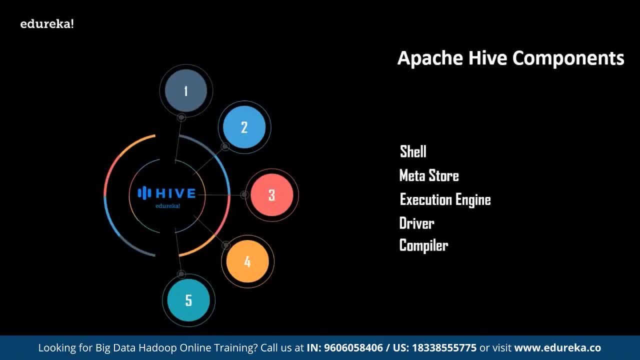 which makes the hive a very editable of a tool. So it starts with the innermost shell. So people who have been using python or any other interpreter based programming language know what is a shell. So it is basically a single line executor where commands are executed. 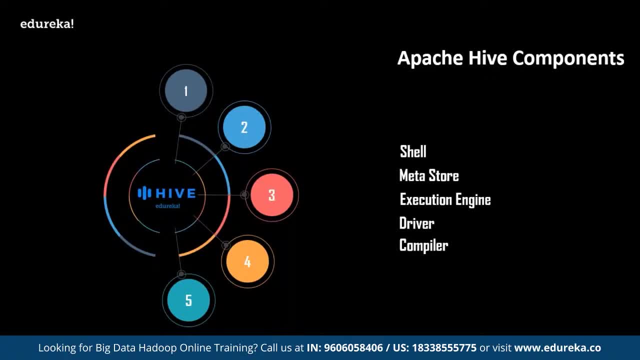 Then comes your Metastore, where the data, what you are getting, is in a format which can be consumed. then is your execution engine, which is a layer which helps you to execute, and this is where the machine level programming- to your application programming- also gets re-orchestrated. 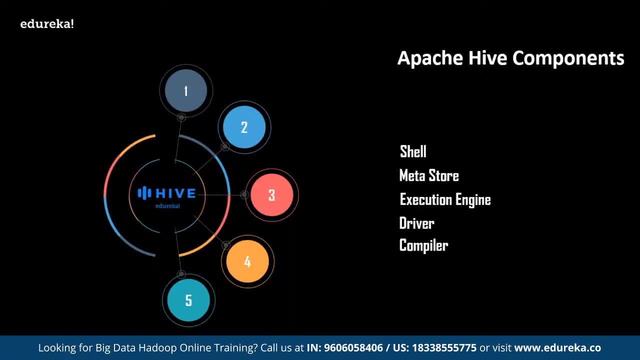 the driver, which acts as a connecting layer, the compiler basically compiles The code. that way, this five components are your Apache hive component. Then, if we have to see the whole thing, basically if we can generate any of the upstream data right, like your Facebook data,